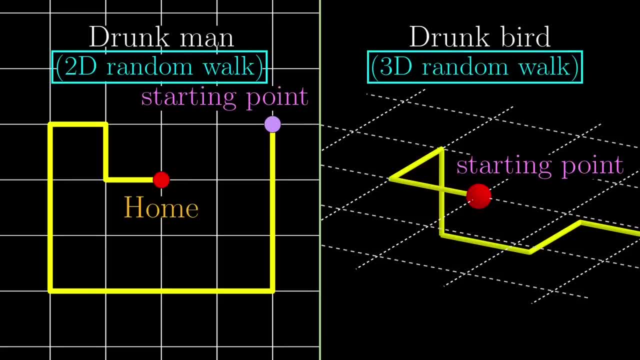 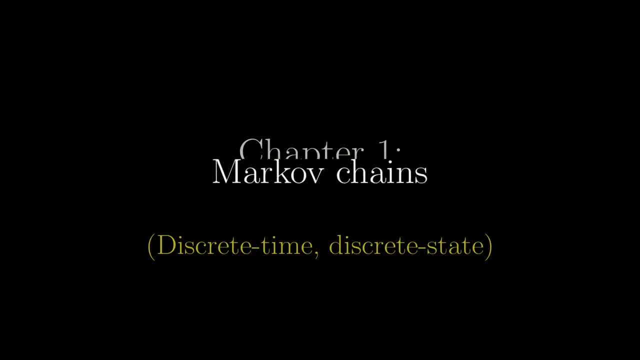 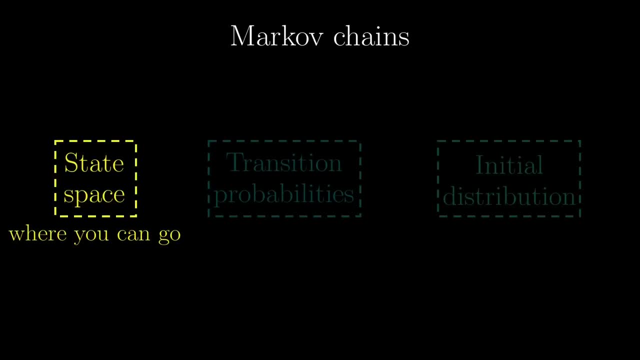 To answer this question, we use the framework of Markov chains. A Markov chain consists of three things. The first is the state space, essentially meaning where you can go In the case of random walks, for simplicity, the state space would be just. 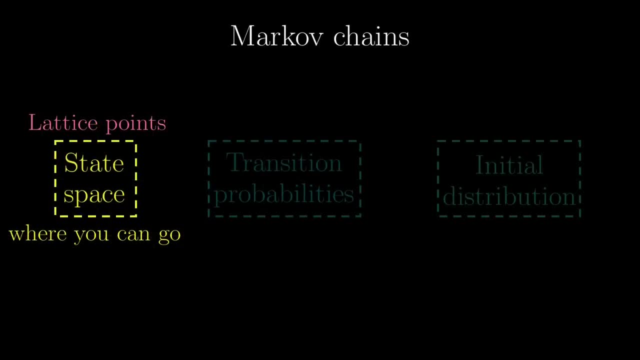 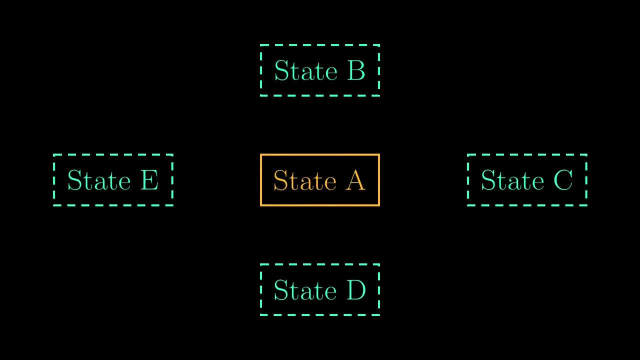 those lattice points. so the drunk man or bird can only visit those lattice points. Second thing is the transition mode, probabilities, because Markov chains are not static. Let's say you are now at state A with four other neighbouring states in the state space. In your next step you can transition to. 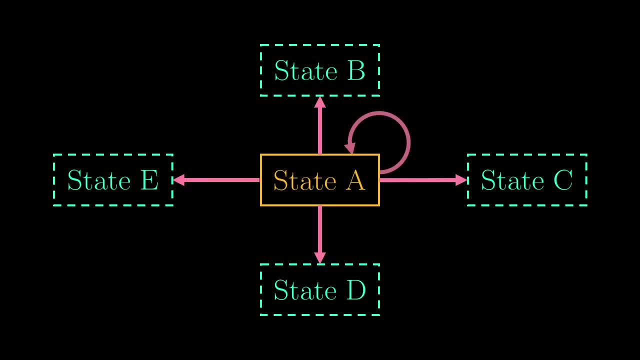 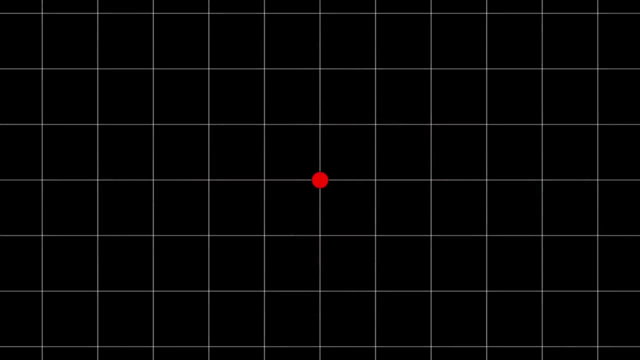 any other states and in general, you might also go back to itself, depending on your setup. For each possible transition, we just assign a probability to it. They are the transition walk. each state has four neighbours and because we have no bias towards any direction, 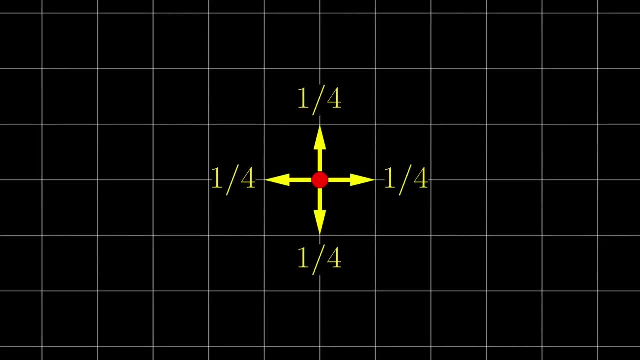 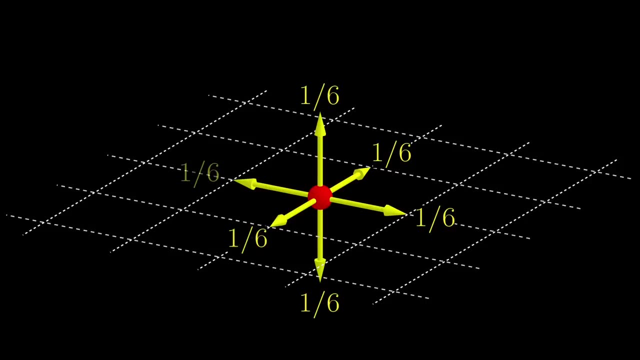 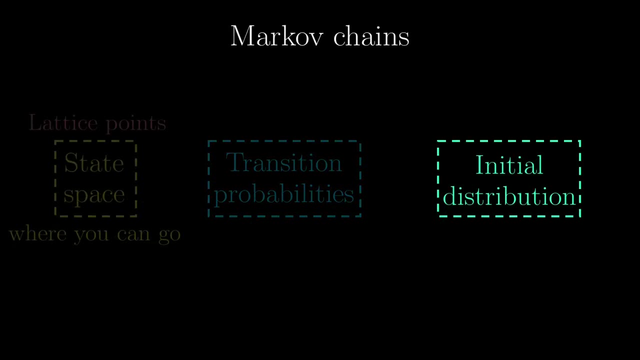 the transition probabilities are all one quarter. Similarly, for a 3D random walk, each state has six neighbours and so the transition probabilities are all one-sixth. The final thing is the initial distribution In a general Markov chain. you have the freedom to. 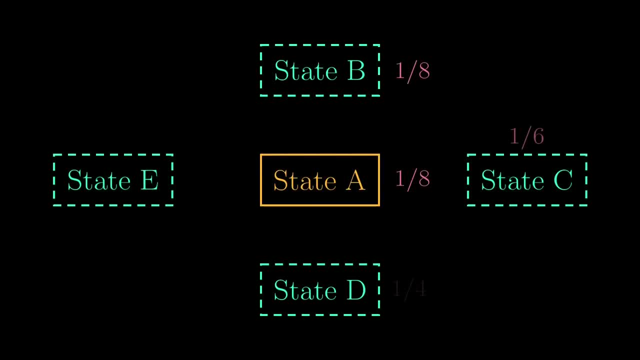 choose which state to start, and so we can assign a probability to it. You can assign a probability to each state indicating how likely you are to start at that state In the case of a random walk. we want to definitively start at the origin, ie a probability. 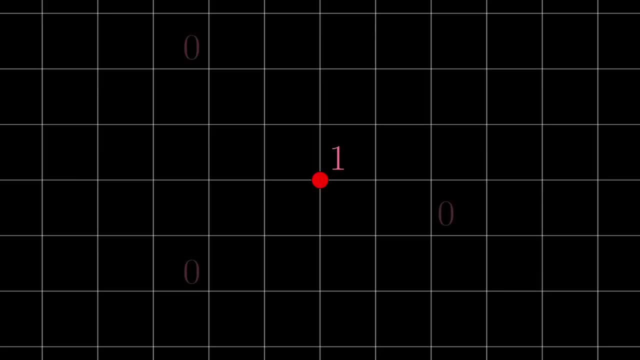 1 of starting at the origin and 0 everywhere else. Wait, didn't you say it doesn't matter where you started? for the 2D case, Don't worry, I'll get there in a minute. These are the three elements in the Markov chain, but there is one key, and that is the probability of starting at the 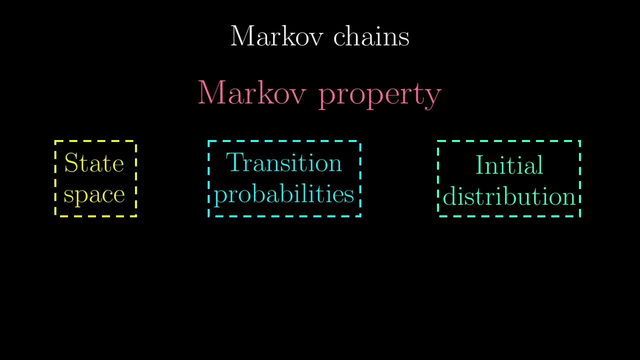 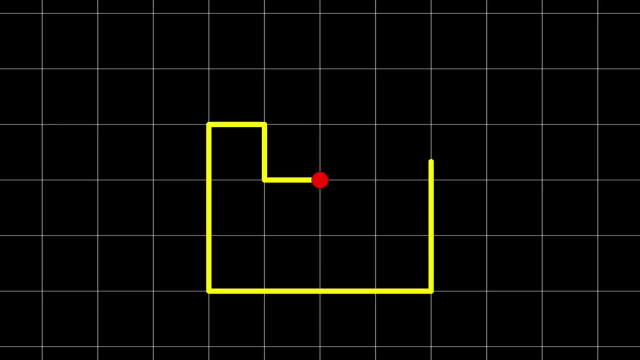 origin. This is the feature that makes it a Markov chain: the Markov property. This is a simple idea that once you have gone to a particular state, you should have already forgotten how you get there and consider the transition probabilities from there without caring about the route that takes. 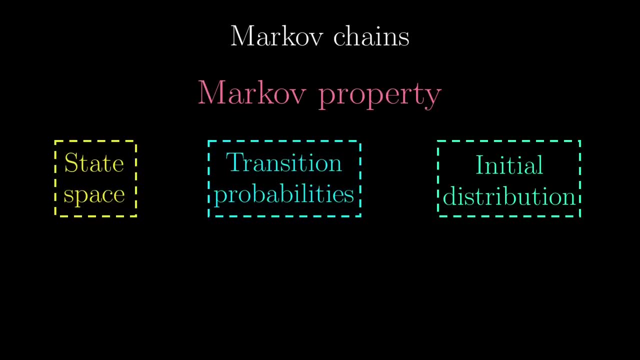 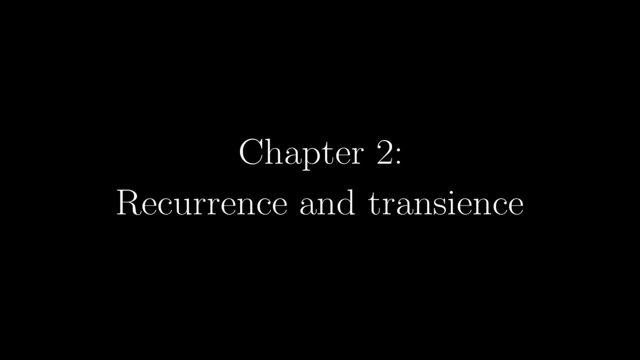 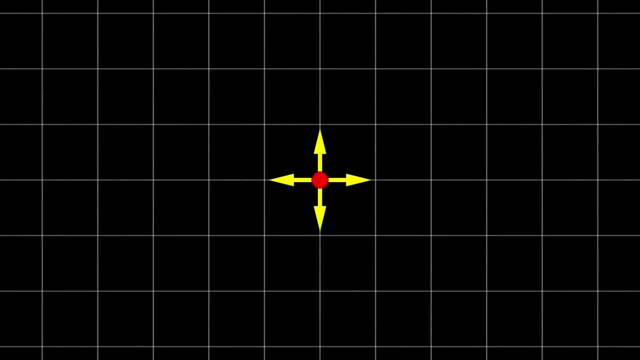 Even that, a random walk is random and every time you run it it gives different results. what can we say about that? One thing we can say is whether you will revisit the origin, if you started there, If you are guaranteed to go back, or in other words, 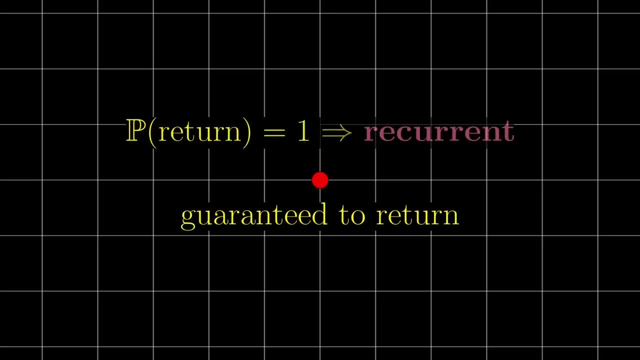 the return probability is 1, then we call that initial state recurrent. If not, then you are not guaranteed to return, and so the return probability is less than 1.. In such a case we call it a transient state, Because you are either guaranteed or not guaranteed to return. 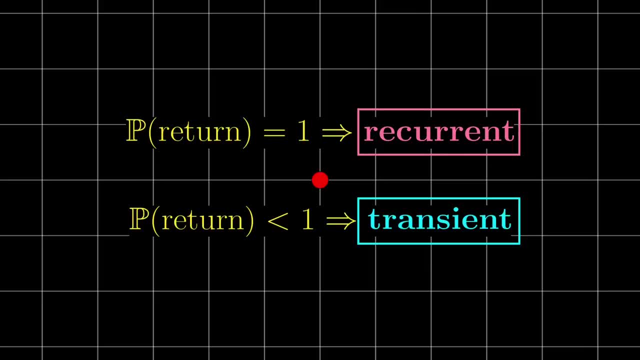 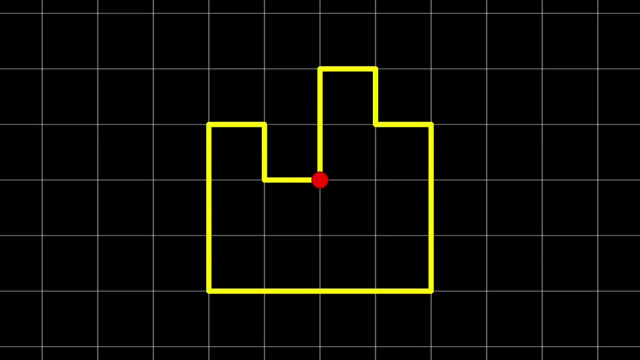 a state is either recurrent or transient. there is no third option. It turns out that in 2D the origin is a recurrent state, and just because this state is recurrent we can already infer that it does not matter where the drunk man started. he will go back to the origin. That takes one or two. 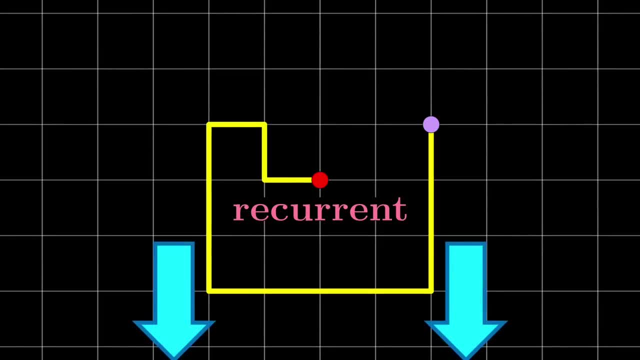 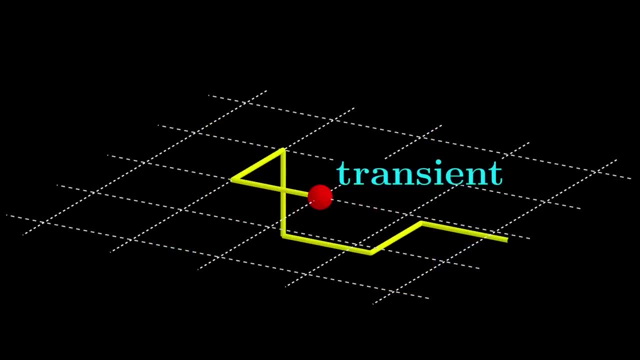 lines of reasoning. On the other hand, the origin in the 3D random walk is a transient state, so the drunk bird may never return. The problem now is how to determine that return probability. Here's the trick. We consider a quantity, v, which is the number of returns to the origin, The implicit 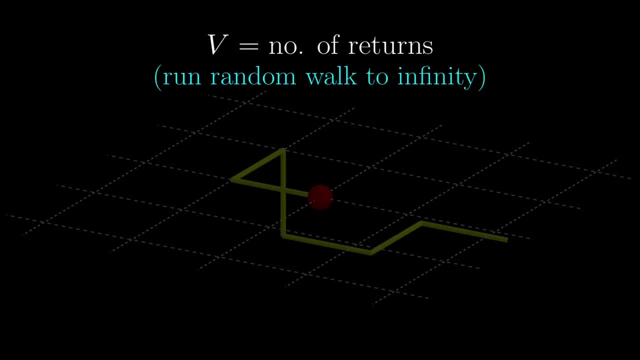 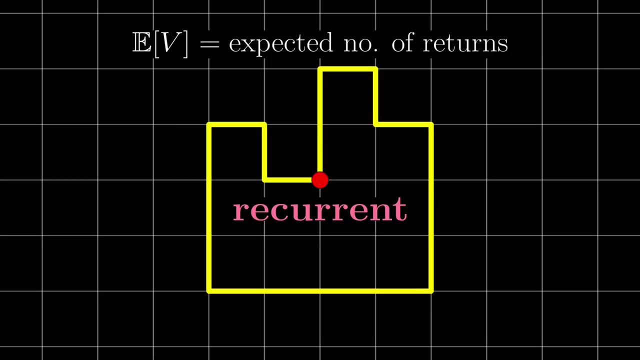 assumption is to run the random walk to infinity, even if you have returned. Our focus, however, is the expectation of v? ie, the expected number of returns. Now for the recurrent case, we are guaranteed to go back, but if we continue to run the random walk by the Markov? 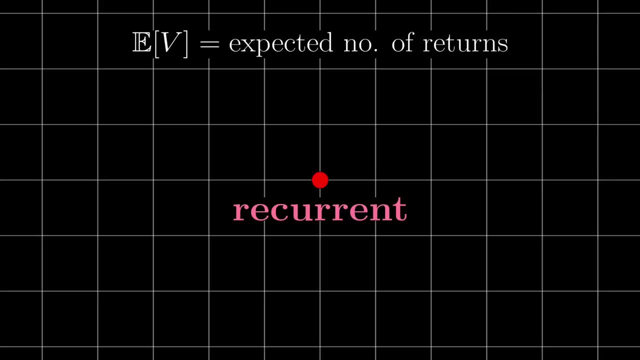 property. we should have forgotten that we have returned, and then we will for sure return to the origin again and again. So the number of returns, v, is guaranteed to be infinite and the expectation would also be infinite. So in this case the expectation of v is the expected number. 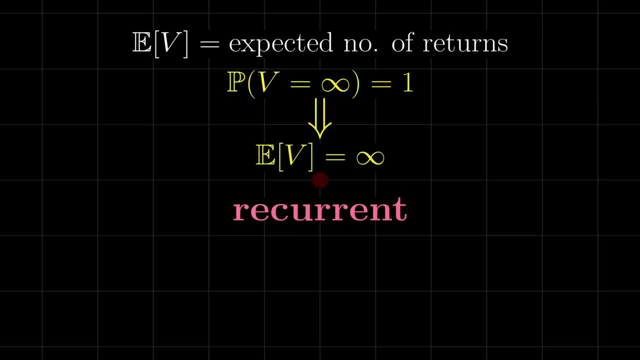 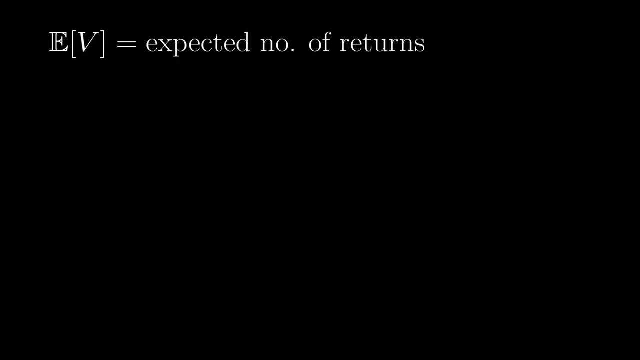 of returns, That is, when the state is recurrent. What if the state is transient? Here is a very clever general trick. By definition, the expectation is 0 times the probability that v is 0,, plus 1 times the probability that v is 1, and so on. But what if we write, for instance, this: 2 times: 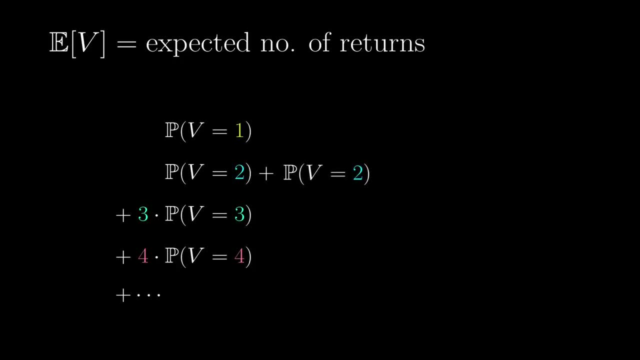 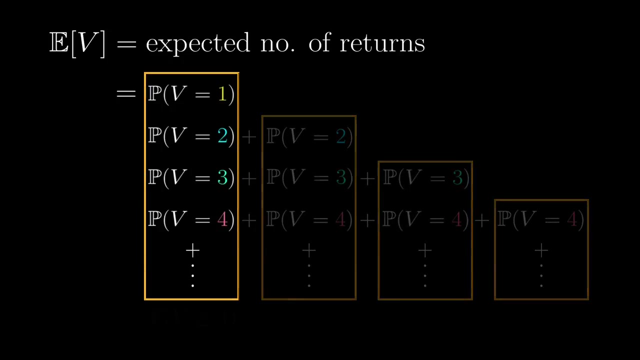 probability as actually the sum of two copies and also do this similarly for the other terms in this sum, Then instead of summing these row by row, we can sum these column by column. For the first column, it is exactly the probability that v is at least 1.. Similarly, 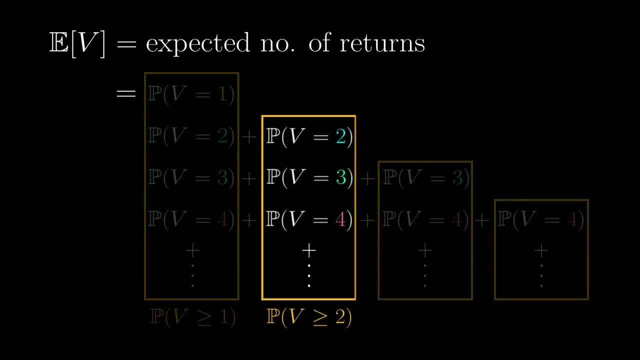 the next column gives the probability that v is at least 2, and so on. The reason this method is useful is that if v is at least 1,, that exactly means you return to the origin at some point, and so this is actually the return probability, And for simplicity we denote it as r. 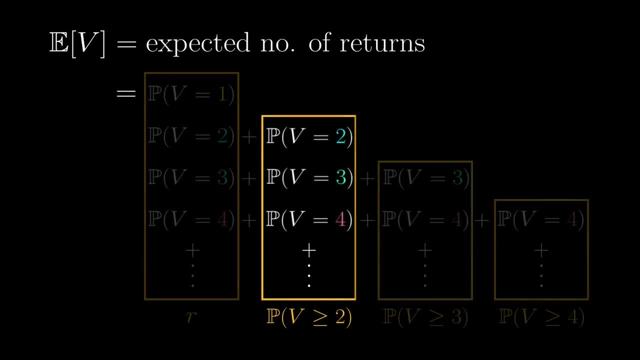 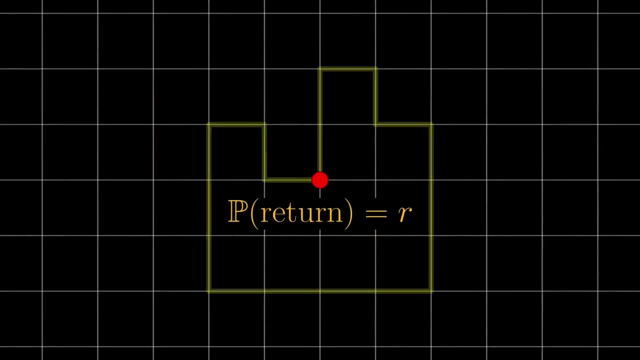 What about the probability of returning at least twice? Well, the probability that you will return is r, but again by the Markov property. you should forget that you have returned, and so the probability that you return again is to multiply by another r And in general, 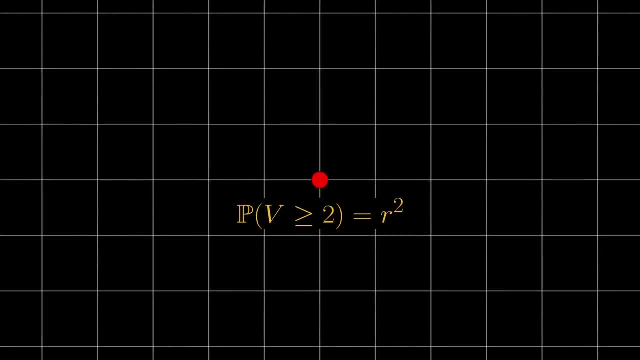 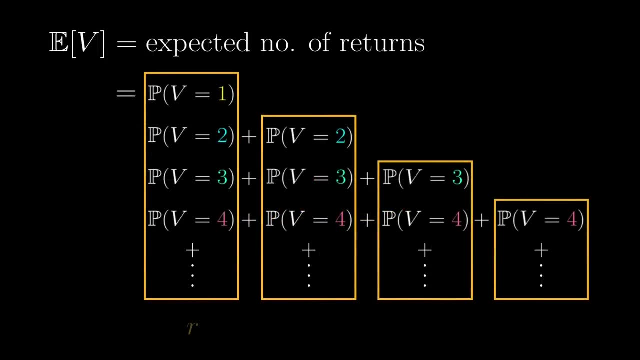 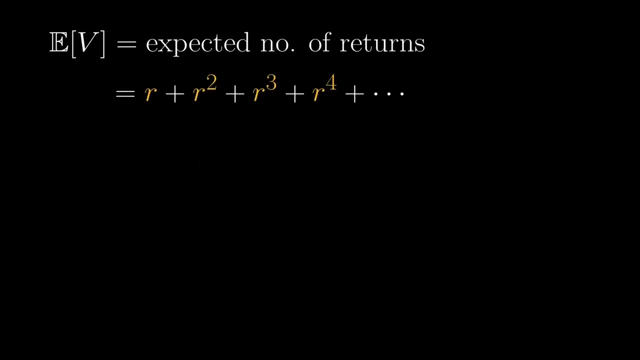 the probability of returning at least k times is r to the k. So if we go back to the expectation, each column actually sums up to a power of r and the expectation is a geometric series. So we know what this should sum to if that return. 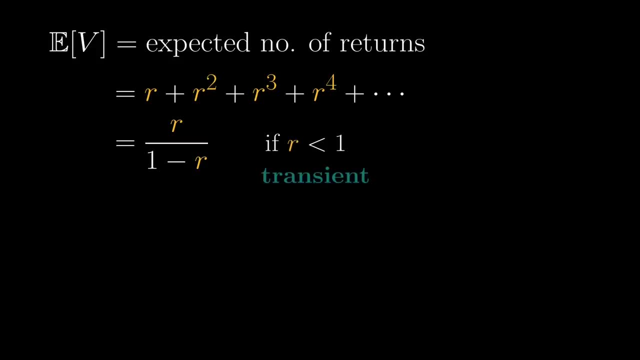 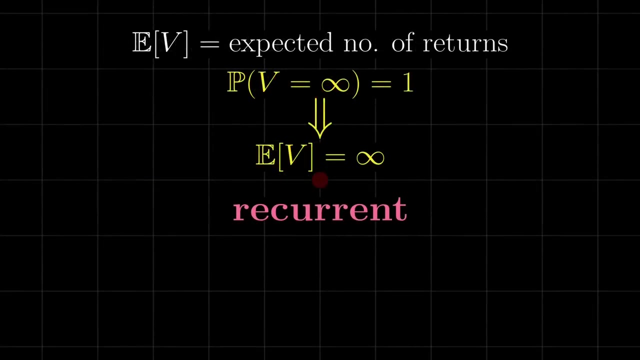 probability is less than 1, which is precisely the case when the state is transient. For now, we only need to know that this is finite if r is less than 1.. However, we have also deduced that for a recurrent state, this expected number of returns is infinite. 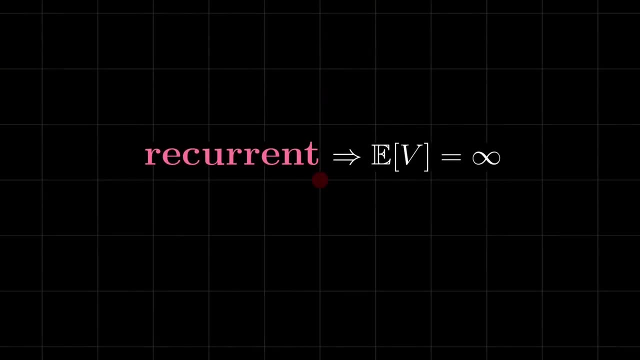 So if the state is recurrent, we have the expectation to be infinite, and if the state is transient the expectation is finite, Because a state is either recurrent or transient. no third option. if say the expectation is infinite, the state could not. 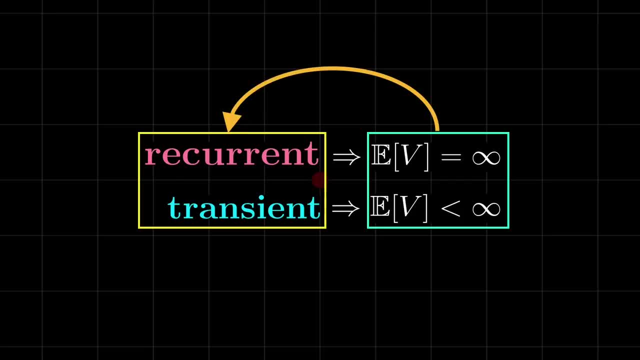 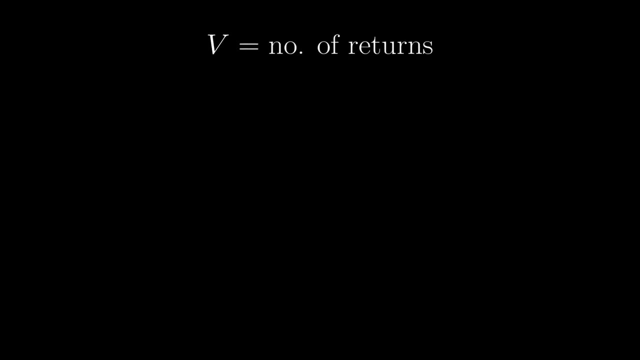 possibly have been transient. So if we know that what the state of r is is notintопрос, we would be getting a result, also called a loss. So if we know whether this expectation is infinite, we are done. Then there is another way of thinking about v? ie rural in speech. the number of returns N. 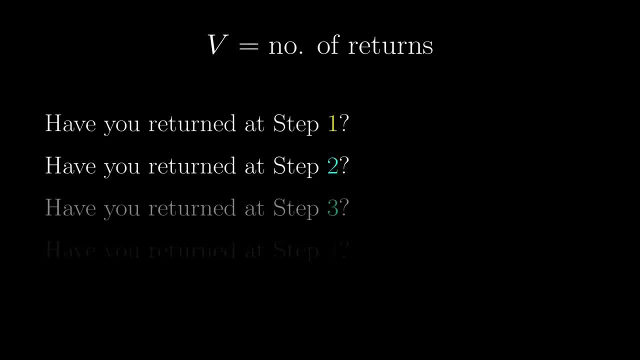 As we come to the end of our work, we first ask ourselves: have we returned at step N? If so, we give it a readout and the results immediately become teasing. Then we add 1 to the tally, And if we don't do so, we don't get braking. the state of r. If we do, then if we do, then we have to do anything to it. If we are at the end of our work, then we conclude that we returned 1 to the state of n. the return is not Tammy next to none, So we end up at the release every 1 cell. So if we enter only 1 in the statement, 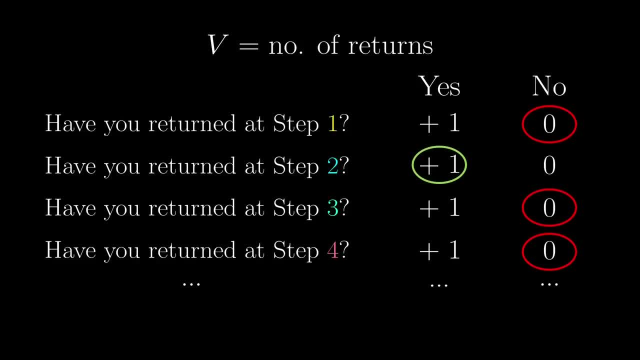 we answered all these questions. we add up the total and we obtain v by just adding up all these plus ones. If we are asking for the expected value of v, we add up the expected value of the first question, the expected value of the second question, and so on. The 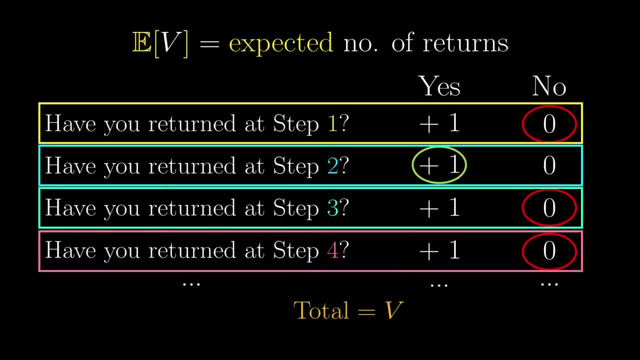 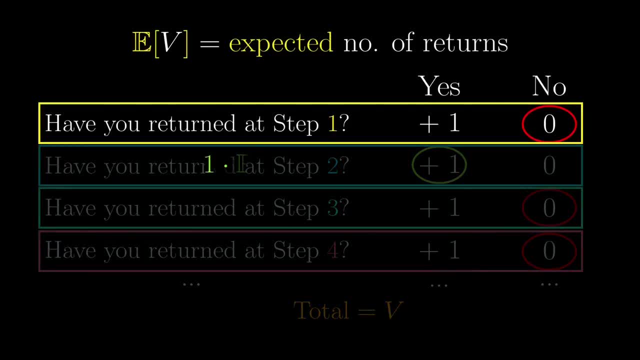 expected value of these yes-no questions are much easier to handle. The expected value of this question would be, by definition, 1 times the probability that you answer yes, plus 0 times that you answer no. Well, that's just the probability that you answer yes. 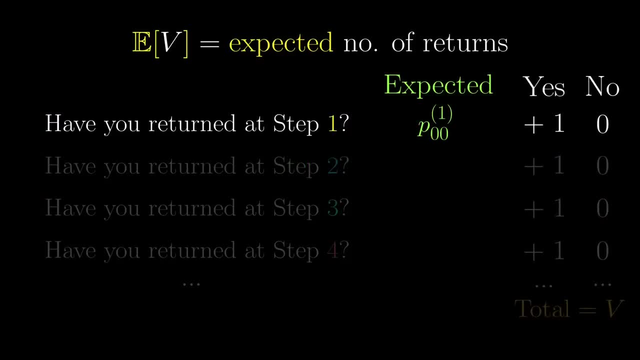 We usually denote this probability as p, with subscript 00 and superscript 1.. The double 0 denotes going from the origin to the origin, ie revisiting the origin, And the superscript just represents the origin At which step you revisit. These probabilities will be the expected value for each question. 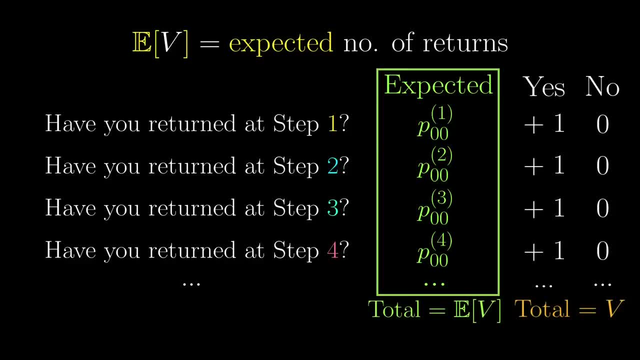 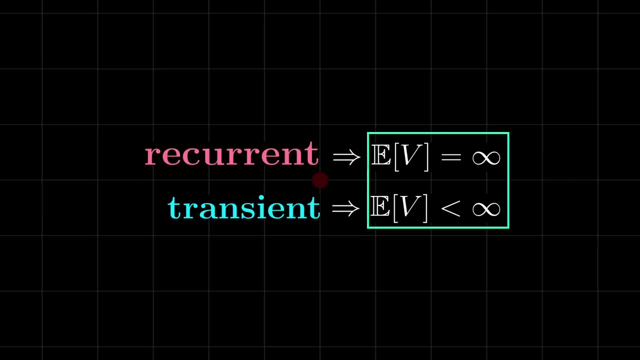 and the sum of these probabilities gives us the expected value of v. So we now have a way of explicitly computing the expected value of v. Previously we deduced that we can simply use the expected value of v to infer whether the state is recurrent, and now we also know. 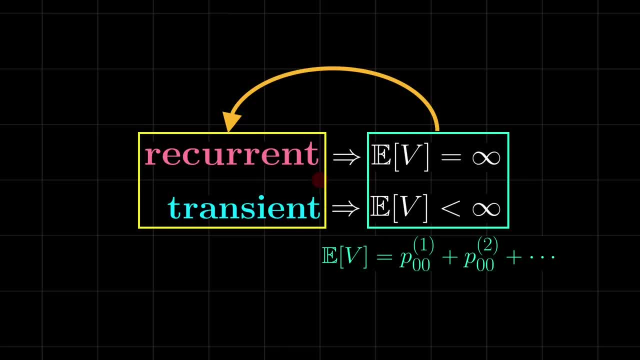 how to explain the expected value of v. So we now have a way of explicitly computing the expected value of v. So once we know whether this series converges, then we know whether the state is recurrent or transient. This whole argument actually works for all Markov chains, including the random walk. we 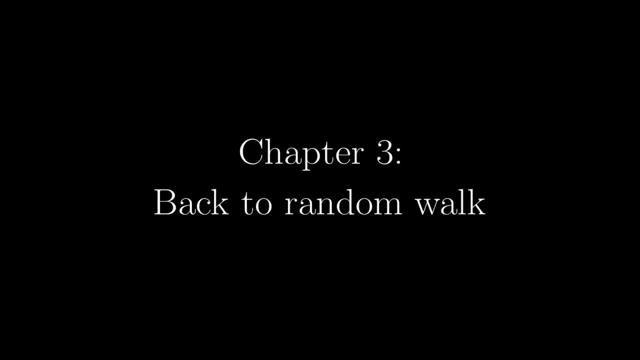 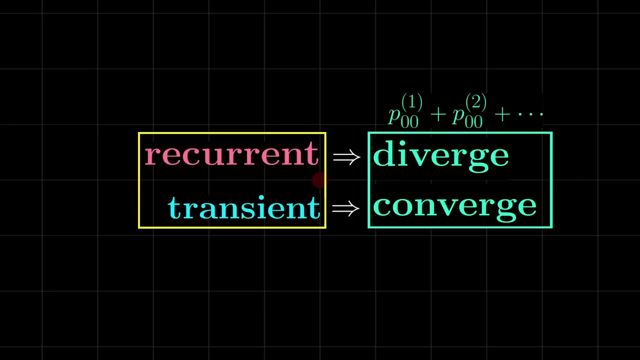 are considering. In the previous chapter we essentially devised a test for recurrence or transient. A 2D random walk is recurrent and a 2D random walk is recurrent and a 2D random walk is transient, So we want to prove that the series diverges. A 3D random walk is transient, so we want 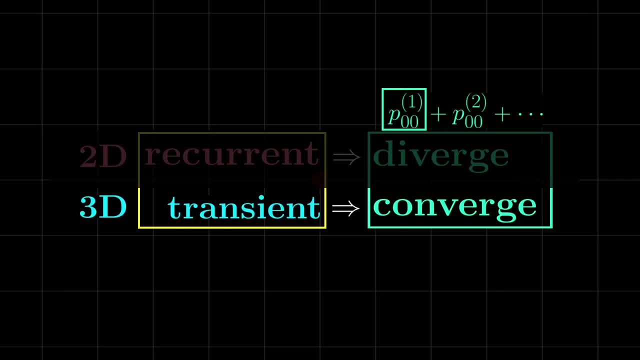 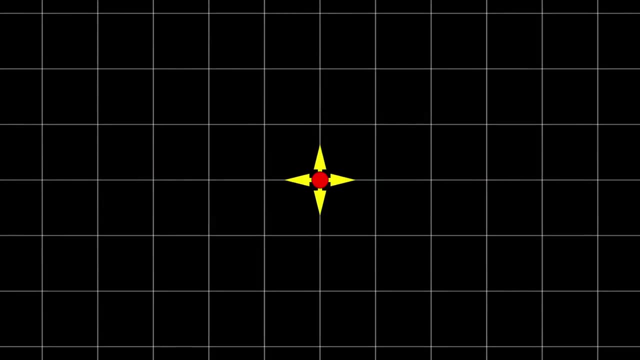 to prove that it converges, But whichever the case, we need to compute each term. In the case of a random walk, you can't possibly go back to the origin after one step, and so this probability is zero. This should not be too surprising, because any return paths would have the same number of 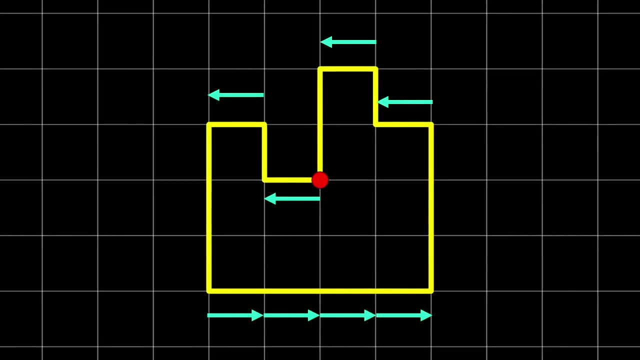 steps to the left as those to the right, and of course, the same number of steps to the right as those to the left, The same number of steps downwards as those upwards, And so the total number of steps here has to be even. So this nth step probability is zero if n is odd, and so we can just focus. 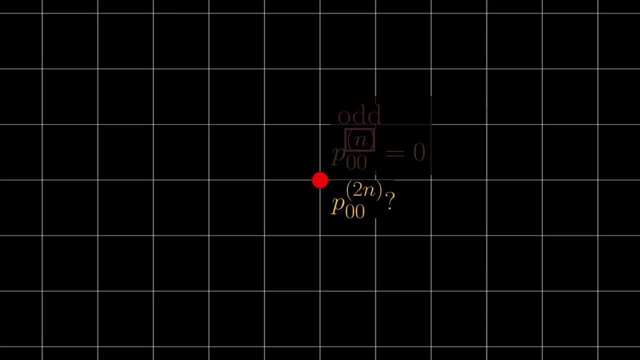 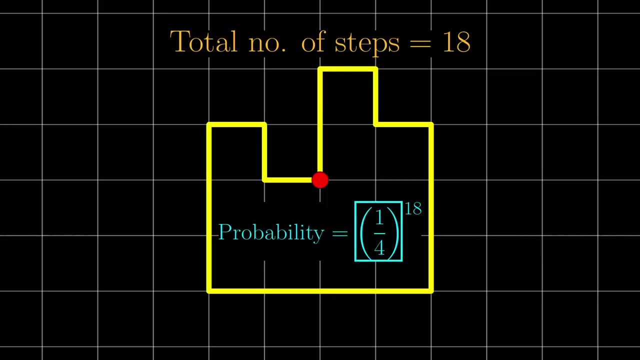 on finding the even two nth step probabilities. Let's say we want a total of 18 steps, then this is a specific possible return path. This specific path has a probability of one quarter Because each step is chosen with probability one quarter and there are 18 steps you need to take. 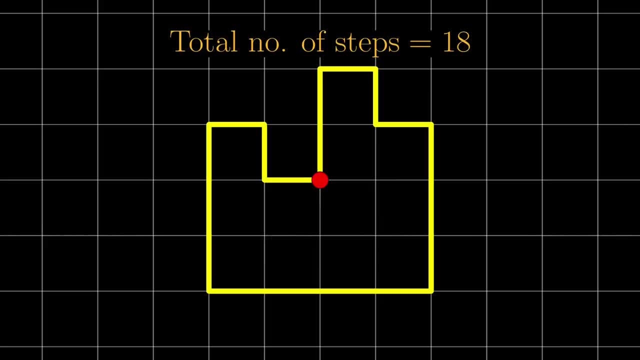 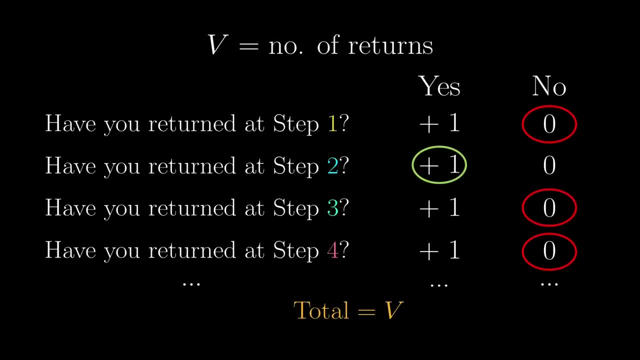 Of course, this is not the only possible path that returns to the origin after 18 steps. This one also does, Even though it has returned to the origin already. as long as you return at step 18, it still counts because you will still answer yes in the previous argument. 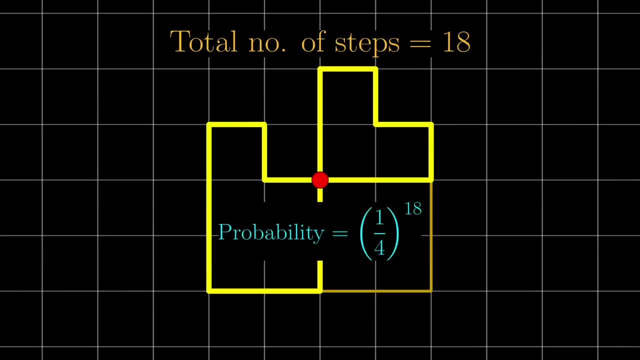 And if you return to the origin after 18 steps, you will return to the origin after 18 steps. And if you return to the origin after 18 steps, you will return to the origin after 18 steps. Anyway, the new path also has probability one quarter to the 18th More explicitly. 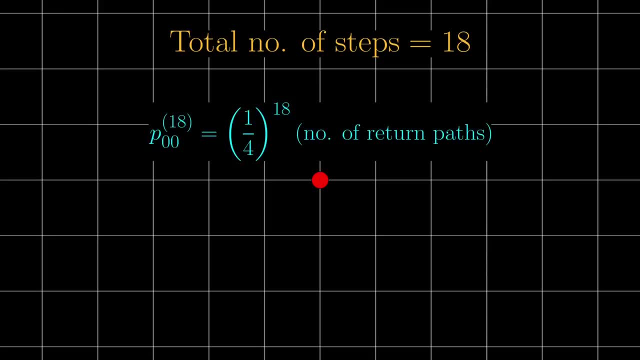 when calculating the 18th step, return probability, we just add up these probabilities- This part is the probability of getting a specific return path- and we then multiply by the number of return paths to get the overall probability. So it all boils down to counting the number of return paths. 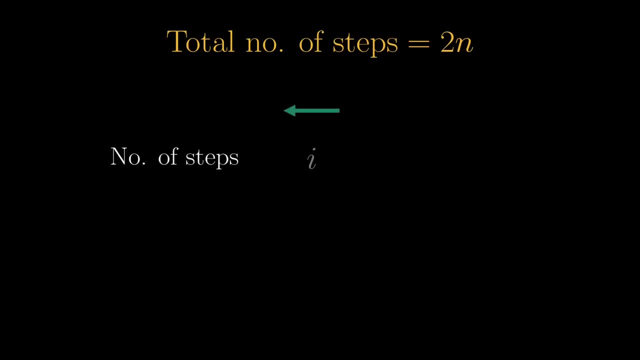 For a total of 2n steps. a return path should have the same number of steps to the left and to the right and the number of steps upwards is the same as downwards. Because the total number of steps is 2n, we can express j in terms of i For a return path. we can imagine it as a sequence of moves. 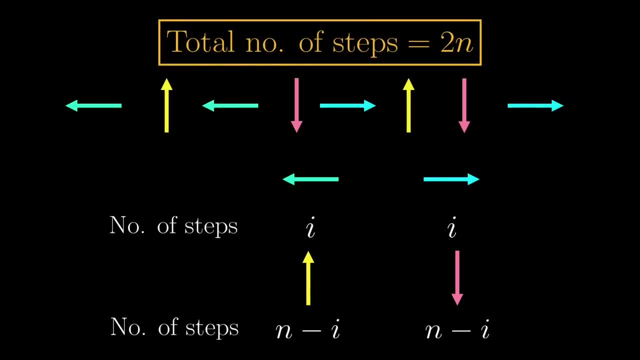 Because there are a total of 2n steps. in total, there are 2n steps, 2n factorial arrangements of these moves. However, if, for example, we just rearrange these two left moves, then the resulting path quite literally hasn't changed. yet it counted. 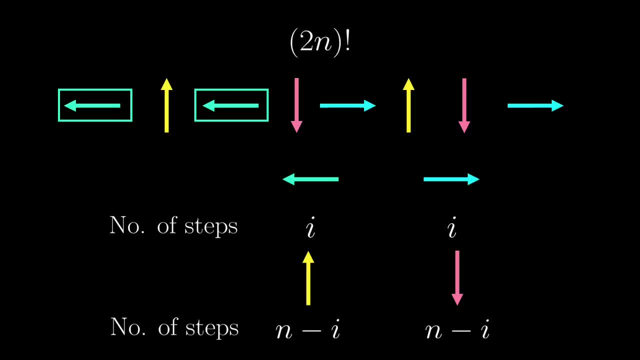 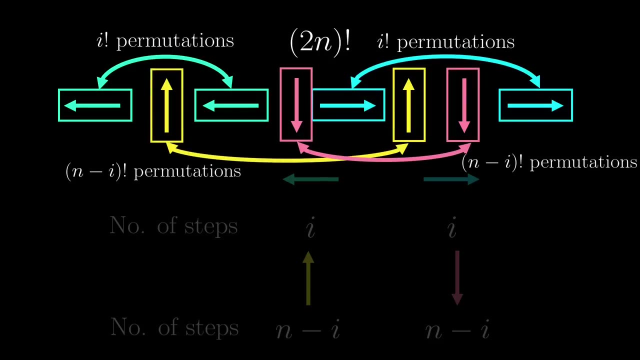 as different in those 2n factorial arrangements Because there are i steps to the left, there are i factorial different permutations in between them And of course the other directions have similar results. These inter-permutations all counted as different in those 2n factorial arrangements. 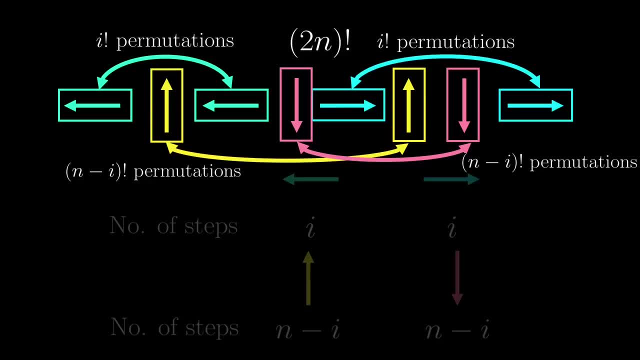 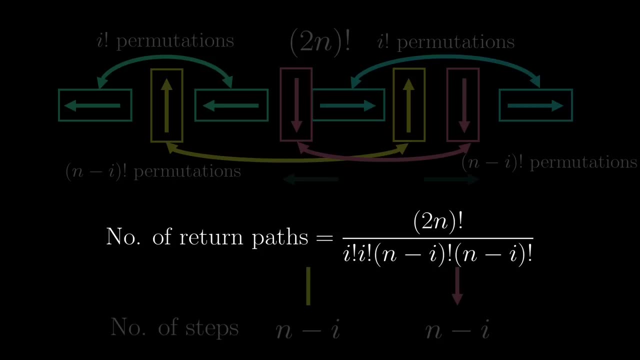 yet they should have been counted the same, And so the number of return paths for a fixed value of i is 2n factorial divided by all these factorials. So, given a value of i, this is the number, and i can range from 0 to n, And so 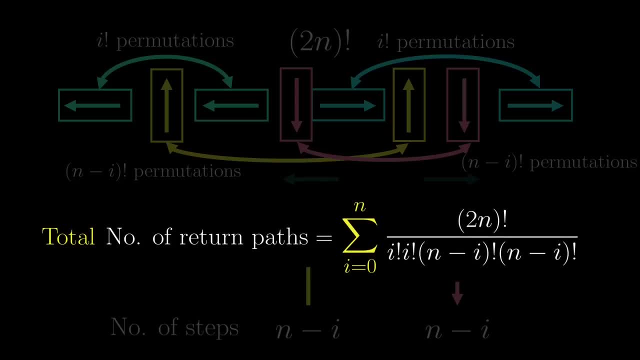 this dual還 is 2n. The final total number of return paths needs to add these up for i, ranging from 0 to n. Finally, this 2n'th steps return probability is ¼ to the 2 n times the total number of. 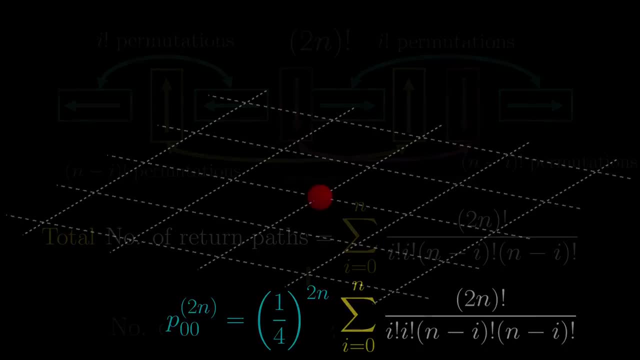 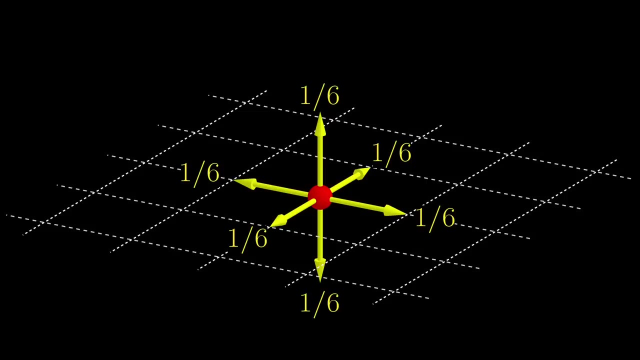 return paths. That's just the case in 2-D. What about 3D, random walk? The only difference is that transition there is one more pair of directions to consider. The two nth step probabilities would be replacing 1 quarter by 1 sixth and for the number of return paths we use a similar method. 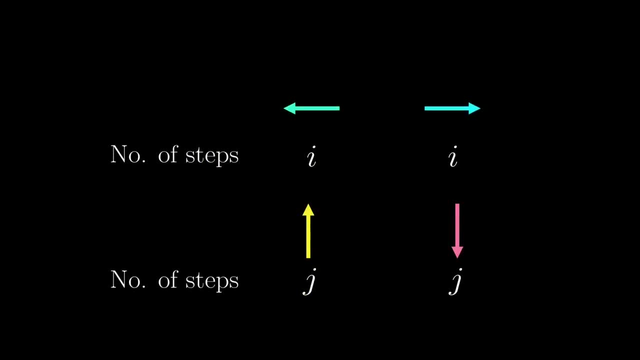 with the only difference being there are three pairs of directions now. So, similarly, for fixed values of i and j, this is the number of return paths, and adding all these for i and j, ranging from 0 to n, will give the total number of return paths. And finally, for the two nth step, 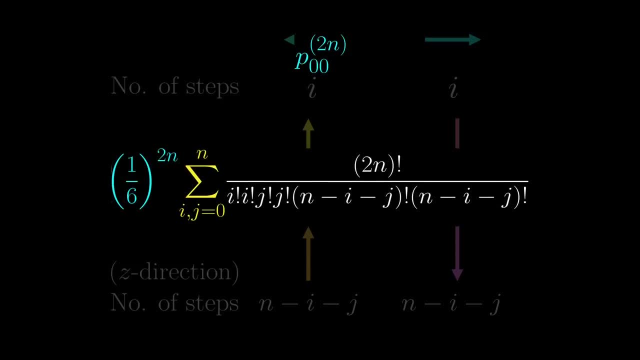 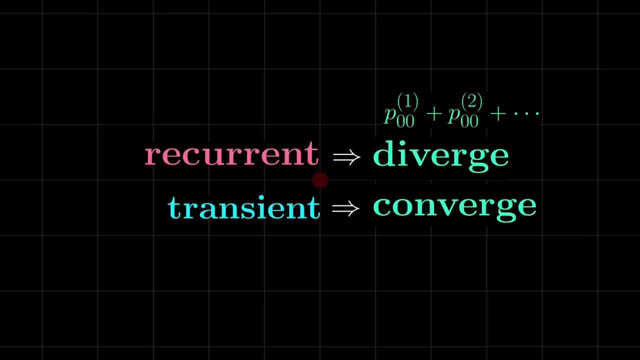 return probability we simply multiply by 1. sixth to the two n. But perhaps it might be useful to remind ourselves why we care about this. We have demonstrated that a state being recurrent or transient implies whether the series diverges or converges. So by knowing whether the series 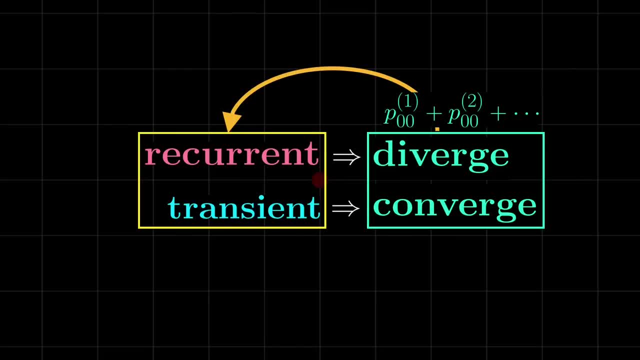 diverges or converges, we can determine whether the state is recurrent or transient And so whether this series converges. we know whether the state is transient. In this chapter we calculated those terms in the series with explicit expressions for the 2D and 3D cases. 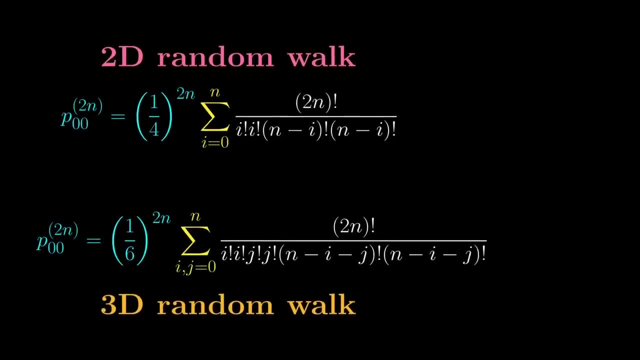 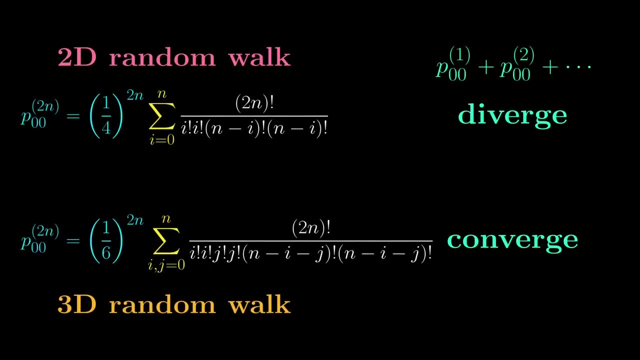 respectively. And what remains is to show that the series formed by the 2D case diverges and the 3D case converges. The very quick reason for it is that each term here scales like 1 over n, so it diverges because the harmonic series diverges And the other term would scale like 1 over n to the 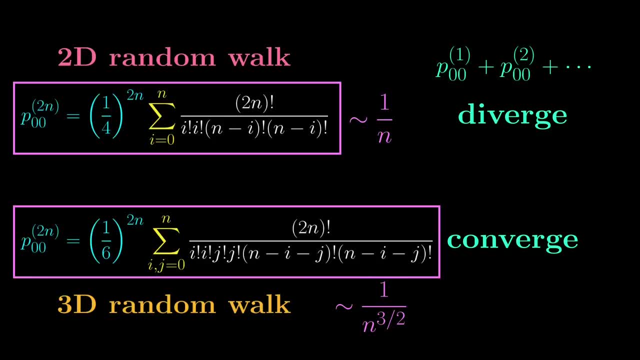 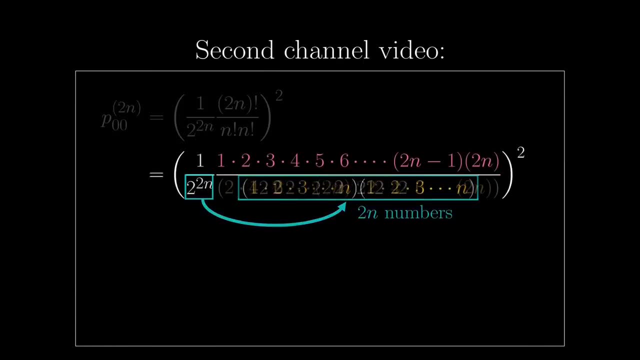 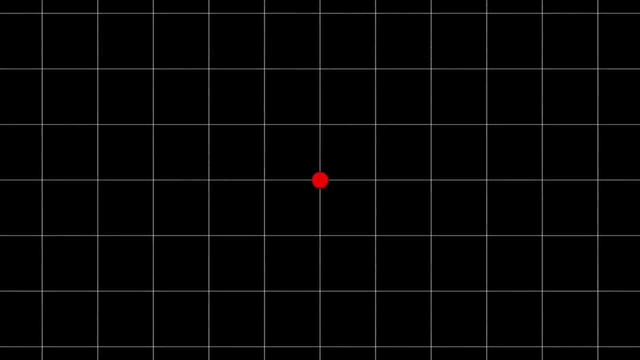 3 halves, and this will lead to a convergent series instead. Originally I wanted to make it into the main video, but this is a bit too much manipulation of expressions and so I ended up making it a second channel video. But I want to give a bit more no-calculation explanation here. We can always think of an.